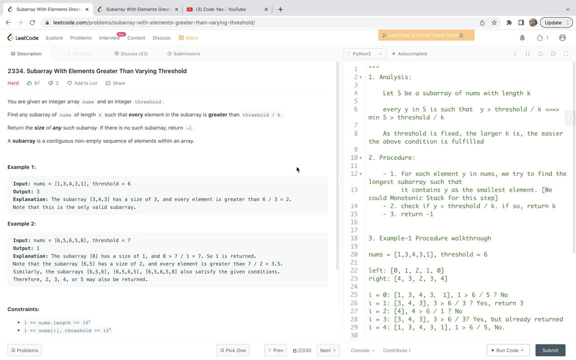 Hello friends, Welcome to my channel. Let's have a look at problem 2334 together: Subarray with elements greater than varying threshold. For this problem we're going to share a stack-based solution. First I'll look at the statement and analyze the problem. 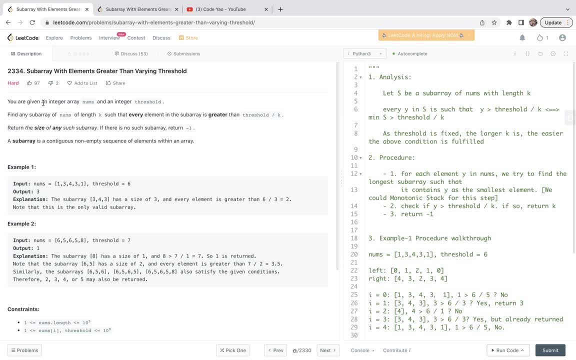 and then we're going to walk through an example with detail and then share the code. First let's look at the statement. We are given an integer array called nums and an integer threshold, So we are required to find any subarray of length k such that every element 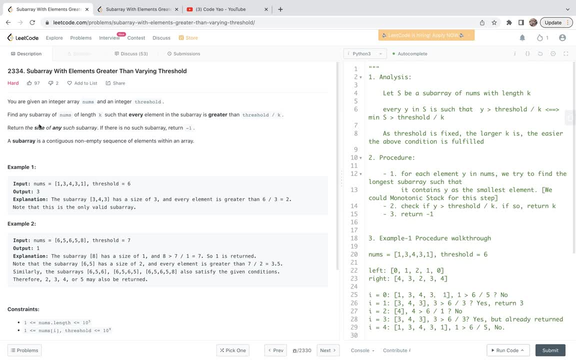 in the subarray is greater than threshold over k. This is the key point in this problem. So we are going to return the size of any such subarray. If there is no such subarray, return negative one. So the next paragraph specifies what's a. 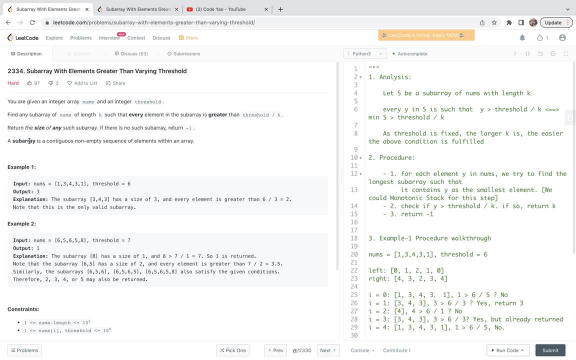 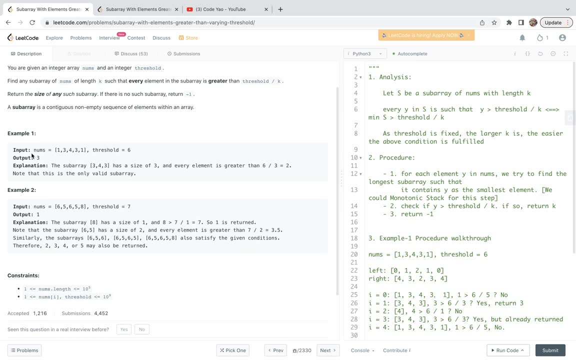 subarray. A subarray is a contiguous, non-empty sequence of elements within an array. So, with that said, let's look at the examples. So, in example one, the threshold value is six and the output is three. So here, three is the size or length of the corresponding 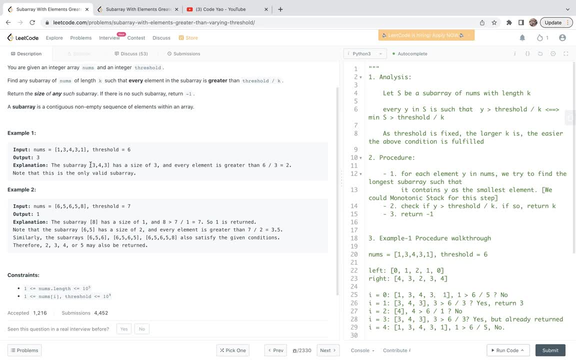 subarray. In the explanation it specifies the subarray which is three, four, three. It has length three and the three so divided. so if we consider six over three, that is two. So every element in three, four, three is greater than two, So the output is three. in example one: 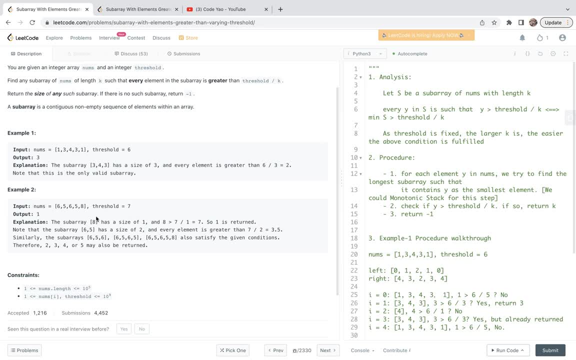 And in example two the threshold value is seven, So the output is one and the corresponding subarray is eight. So this is a single element subarray. Its length is one, So eight is greater than seven over one right. So with that said, 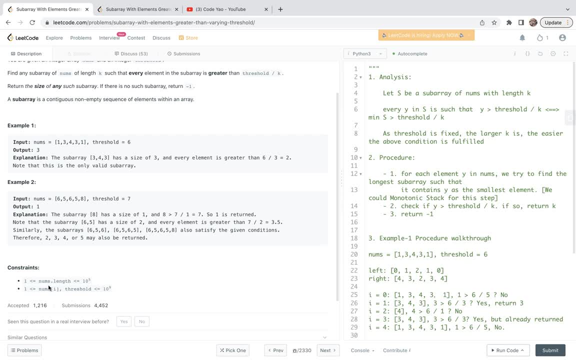 let's look at the constraints of this problem. So the length of the array nums is greater or equal than one, which tells it's not empty, and less or equal than or equal to ten, to the power of nine, This is a large number. So, secondly, the range of nums elements and the threshold value. 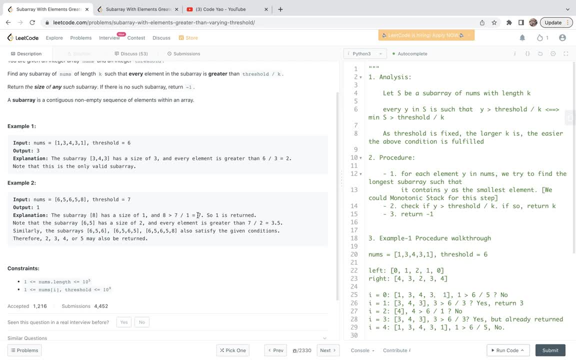 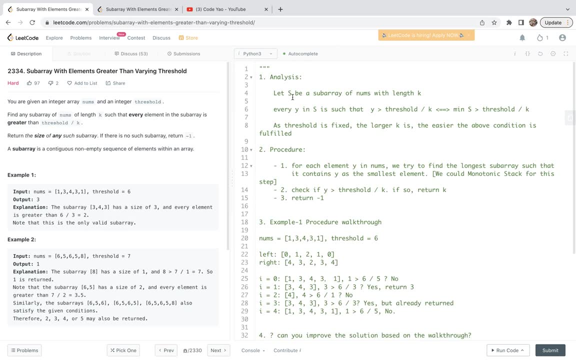 is between one and ten to the power of nine. So, with that said, let's look at the analysis for this problem, So we can consider a such subarray. Let's call it f, So with length, k, So the problem. 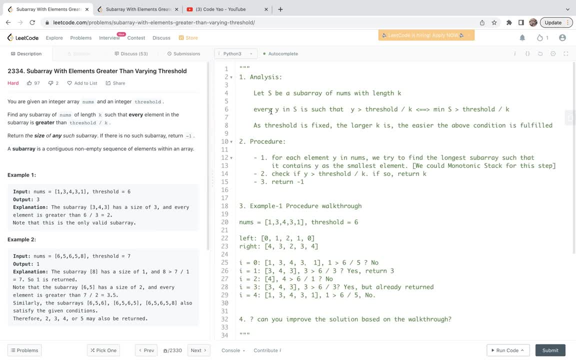 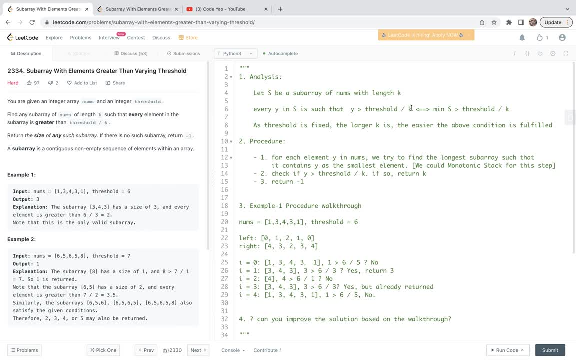 So actually this condition itself is not very straightforward to check, But this statement or condition is equivalent to seeing that the minimum element in S is greater than the threshold value over the length k. So with this point realized, actually the procedure is very straightforward. 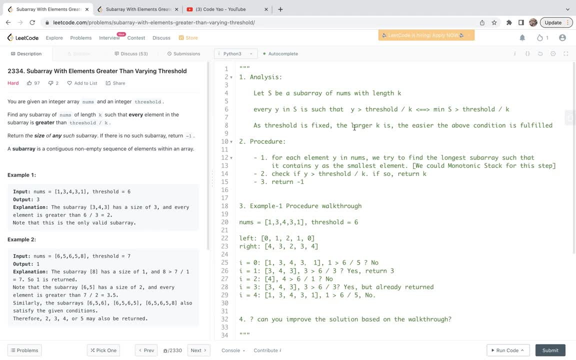 The reason is that the threshold value is fixed. The larger k is, the easier the above condition is fulfilled. So with this equivalence relation we're going to mimic or propose the following procedure. So first, for each element y in nums, we try to find the longest subarray, such that it contains this element y as the smallest element. 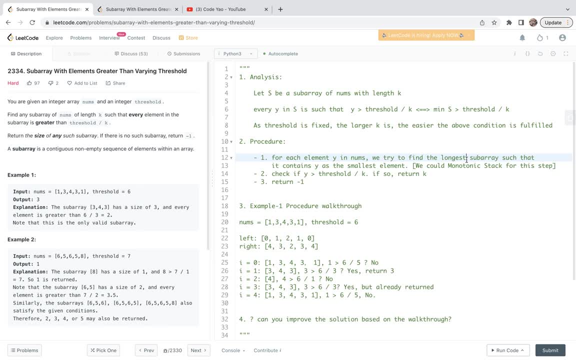 So here longest means that we try to enlarge the length around this number as large as possible. So for this step actually it's a standard monotonic stack operation. So secondly, we check if this y, because this y is the minimum element in the corresponding subarray. 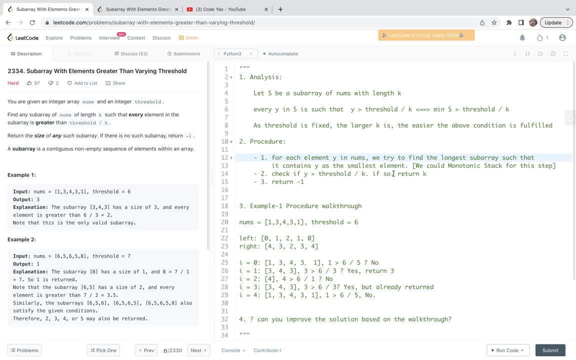 If it's greater than the threshold over the length. if so, we just return the length k. So after this loop, if nothing is already returned, we're going to return negative 1.. All right, So now we can see that the threshold value is fixed according to the assumption or the requirement by the problem statement. 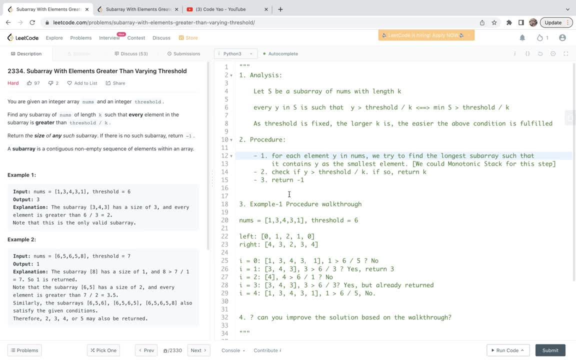 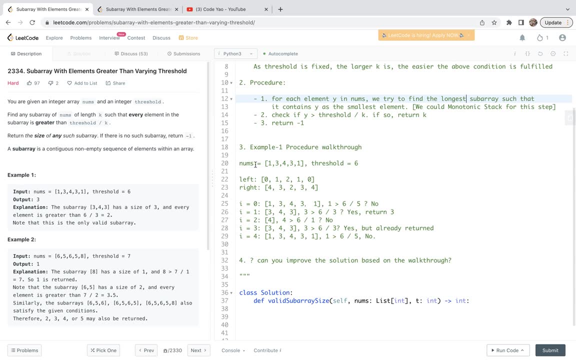 So this actually finishes the analysis and the procedure. So let's look at a specific example to gain the idea. So let's use example 1 to fix this idea. So in example 1, so the threshold value is 6, right? 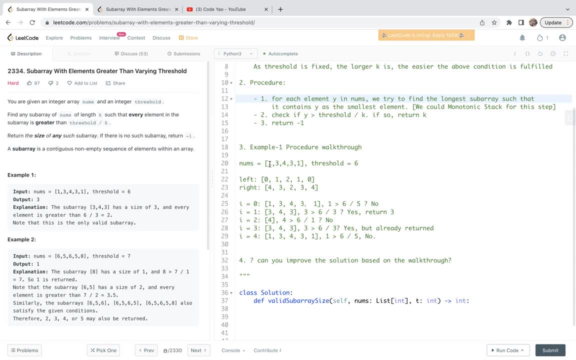 So, in order for each element, see 1 or 3 here For each element in nums- in order to fix or determine the corresponding subarray which contains the element as a minimal element, we just need to specify the left and right boundaries. 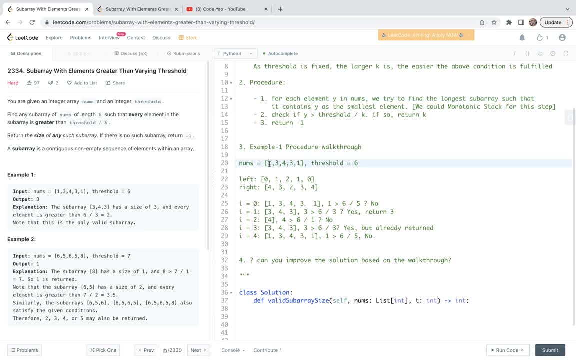 For example, in the i equals 0,, we look at the number 1.. So the corresponding index for left and right boundaries are 0 and 4, respectively, Meaning that so, starting from index 0,, ending at index 1.. 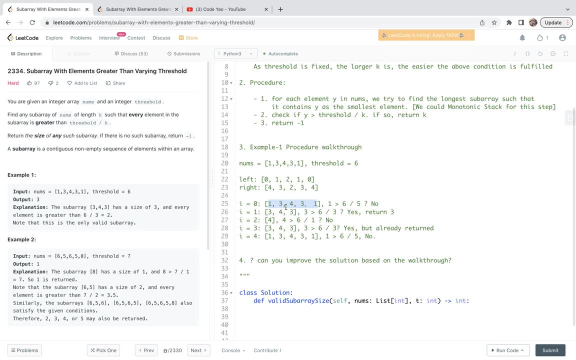 So this corresponding subarray contains this 1.. And also this 1 is the smallest element. Then we are going to check if 1 is greater than the threshold divided by the length. It's not, So we continue. So when we look at the index, i equals 1, the number is 3.. 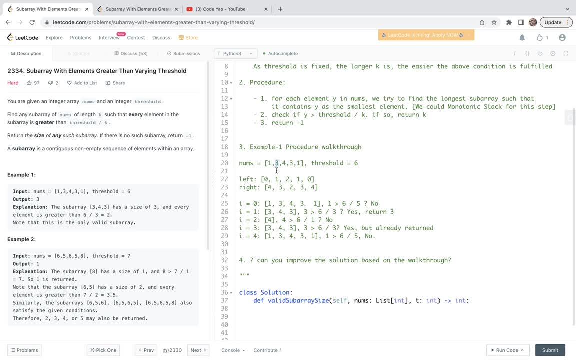 So the corresponding boundaries is 1 and 3.. Meaning that we're looking at 1, 4, 3.. 1, 4, 6, 3, 4, 3.. So this is the corresponding subarray. 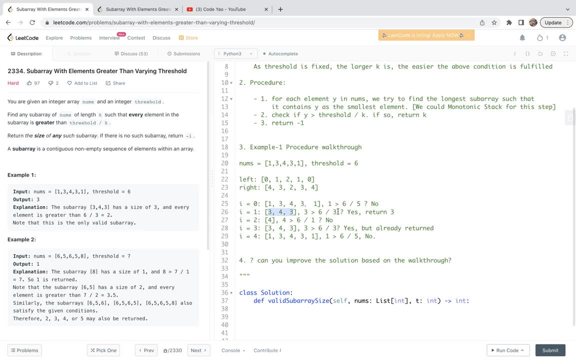 So we check if 3 is greater than 6 over 3.. If so, we're going to return. So here is yes, So we return the size 3.. So up to here, actually, the procedure for this specific example ends. 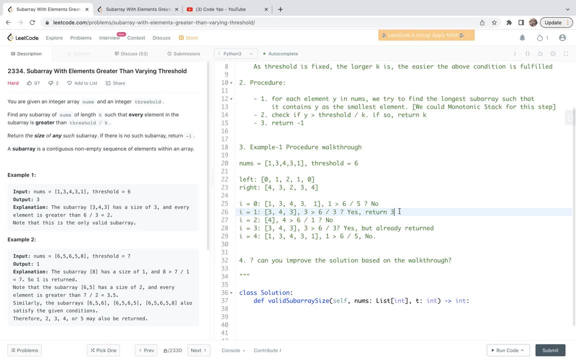 But in order to gain more matching information or intuition, we continue to check for the other elements. So when i equals 2, we're looking at number 4.. So the corresponding index are 2 and 2.. In other words, the subarray is 4 itself, with length 1.. 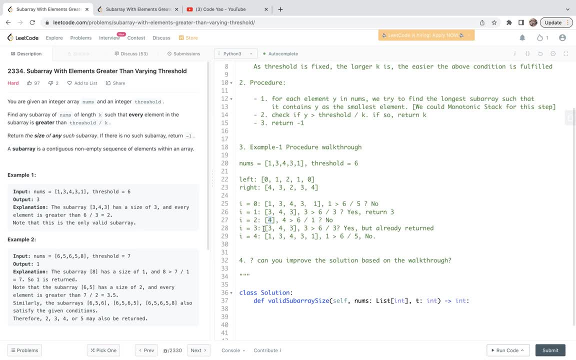 So we check if 4 is greater than 6 over 1. It's no Right. So also let's look at this 3. So this 3 actually equals this 3. So the corresponding subarray is the same as the left and right indices. 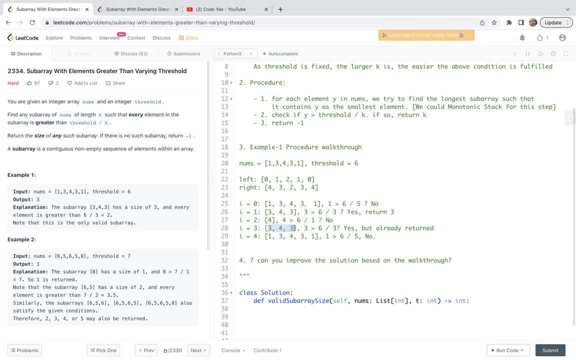 So the corresponding indices or boundaries are the same. So we check 3,, 4, 3.. And 3 is greater than 6 over 3.. Here is yes, But you know we already returned in the step when we're looking at i equals 1.. 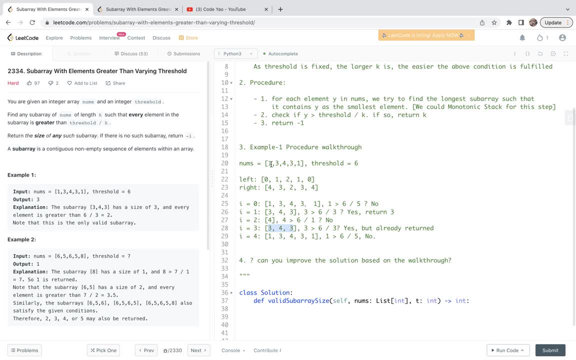 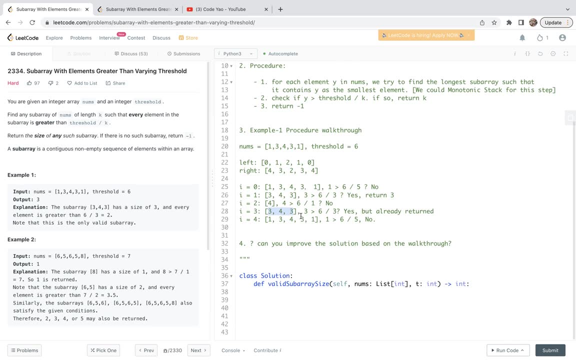 So when i equals 4, we are examining 1 again, right, similar as we examined the first one corresponding to index i equals 0. So, with that said, actually we are ready to share the code For the code. let me first do some preparations and initializations. 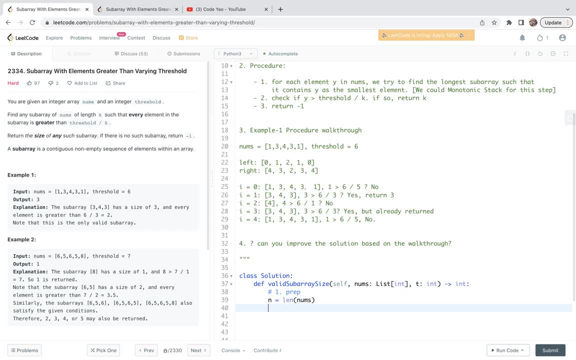 So first I'm going to track the length information for this num- So this is the routine- And then, in order to determine the subarrays corresponding to each number, we're going to determine the left and right boundaries. For this. we are going to do some initialization. 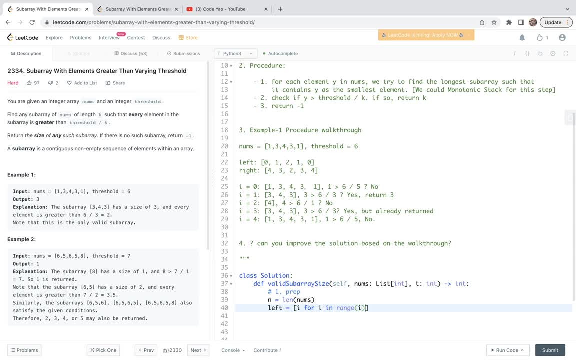 So for left is i for i in range i. So this left will store the corresponding left boundaries for each index or equivalently the corresponding number. Similarly for the right: i for i in range n. So here is n right n is the length we tracked. 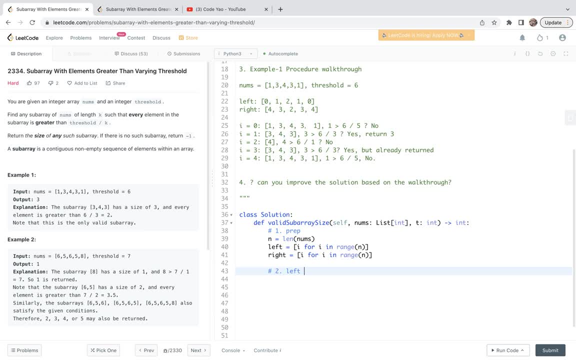 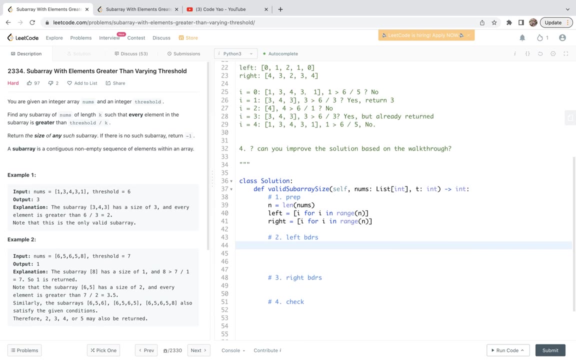 So, with that said, what we want to do is find the left boundaries and find the right boundaries And then do the check right. So let's first fix the left boundaries. For this we are going to initialize a stack because, as we mentioned, 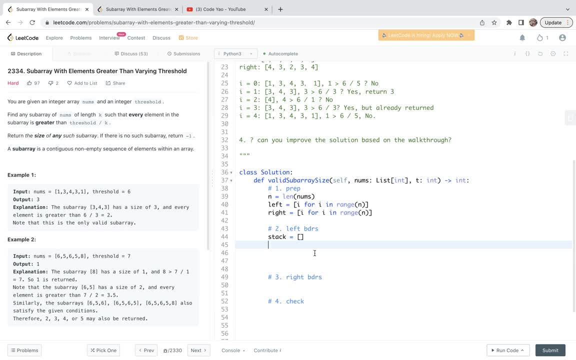 we are going to use the monotonic stack operations. So we are going to determine the left boundary for each number in nums, for i in range m. So then we are going to do the standard monotonic stack operation: Val loops right. 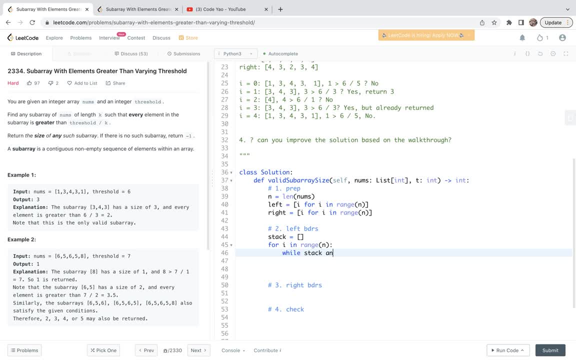 So val stack. So if stack is not empty, we are going to do some pop operations. So we are going to check if nums, the stack top element, is greater or equal than the nums i. right, So we want nums i to be the minimal element in the corresponding subarray. 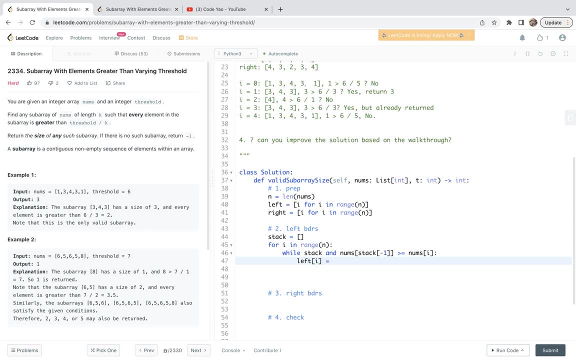 So for this we are going to do some reset continuously. So basically, we are going to reset with the stack top left boundary. So each time we push the left boundary to be as left as possible, right. So here, notice that we need to set as the boundary. 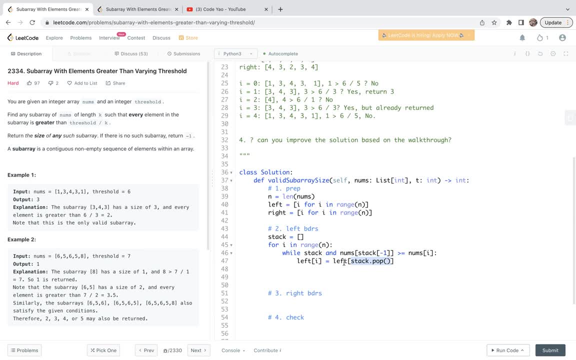 left boundary for the top element in the stack. not setting the left i equals stack pop itself. So this is important, So also this is standard operation. So we are going to append this current index, For example, if the stack is empty, at the very beginning. 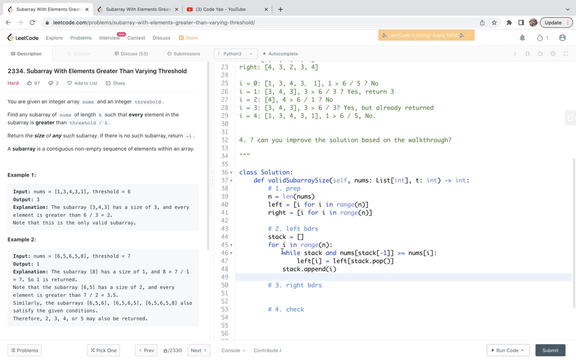 So let's see what motion is for this val loop. So if we exit this val loop, there are two possibilities: Either the stack is empty or the top element in the stack is less than nums i. So this is exactly the stop condition, right? 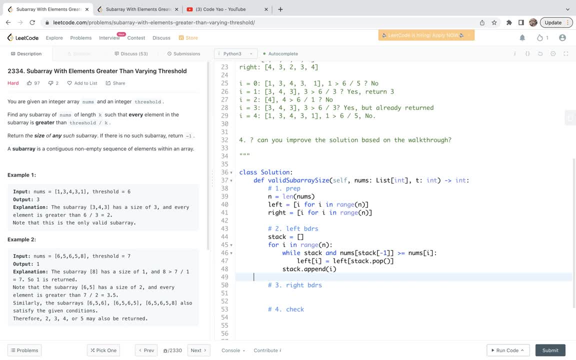 Because we need nums i to be the minimum element. So, with that said, basically we are going to set the right boundary. Essentially, we just copy this one, do some modification. right, So we are using the same name and it's okay. 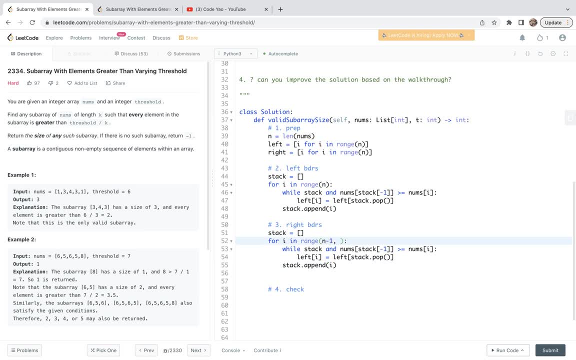 And then for setting the right boundary, we're going to do it reversely, from right to left, So we are ending at the index zero. So we're going to write here negative one And the increment is also negative one Because we are decreasing. 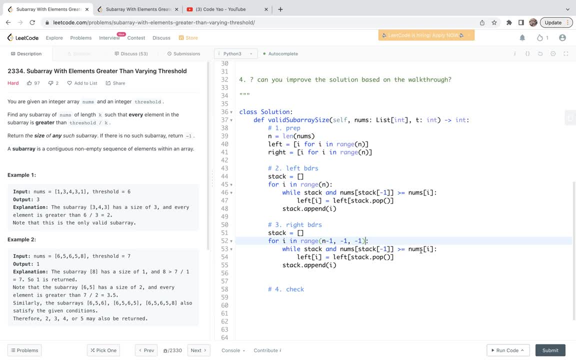 So val, stack and nums i is greater or equal than nums i. This is correct. No modification is needed. But here we're going to change it to be right, right. So this way we have already set the right boundaries. So now we're going to do the check. 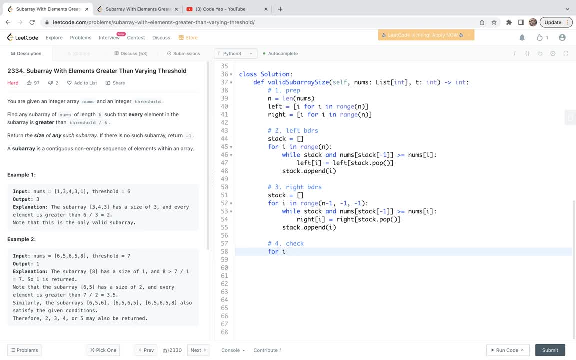 So this is actually very routine. So we're going to, We're going to reverse the nums list. Then the corresponding number is, of course, on nums i And the corresponding subarray containing this: nums i as the minimum element has says reg i minus left i. 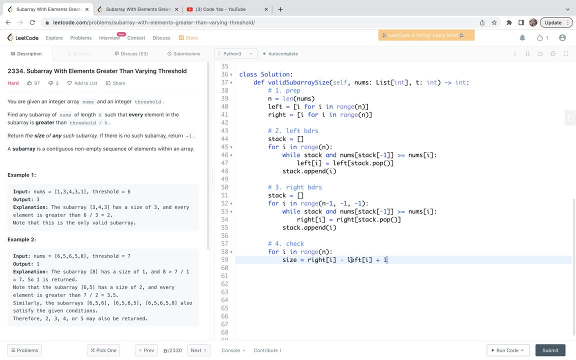 Don't forget the plus one, Because reg i is the end index and left i is the beginning index, Both inclusive. So we are computing the set by the index difference plus one. Then we're going to check the condition. So if the nums i is greater than t, over this set, right. 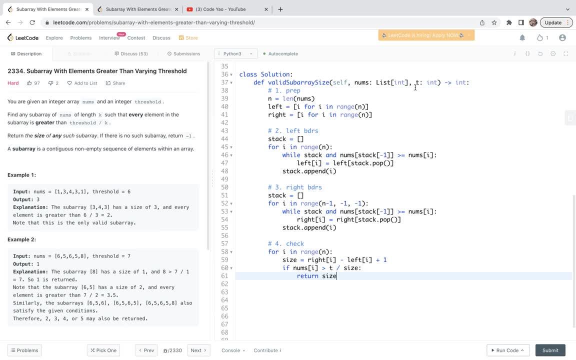 If so, we are going to return the set. So here t is a threshold value. So I have changed this threshold value argument in the original function signature as t for convenience. So if after this loop nothing returned, we're going to return negative one. 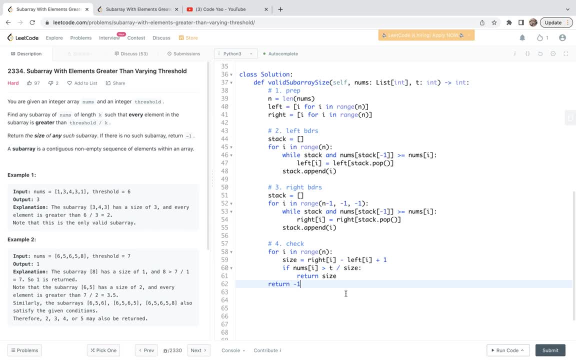 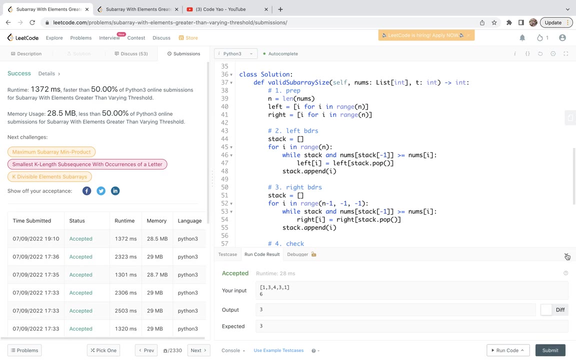 Right, So this is the full code for this problem. Let's do a simple check for special case. It passes the special case. Let's do a generic case check. Yeah, it passes the generic case check. So for this problem here. 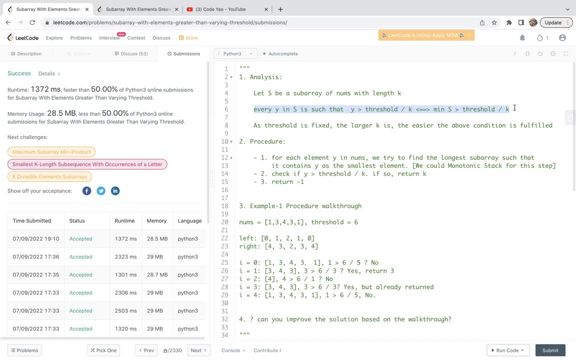 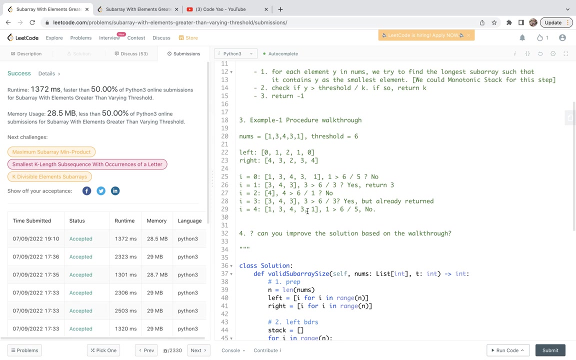 here, at the point, this point, the equivalence is the key. So once we realize the equivalence here, so it leads to the following procedure in step two: directly. And however, this solution we provide here is sort of brute force, in the sense that we checked this: left boundaries and right boundaries for all the numbers.